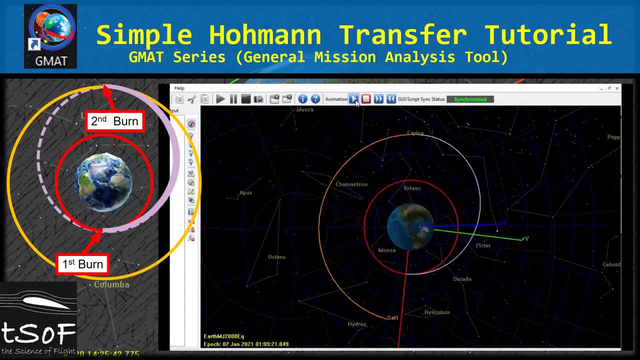 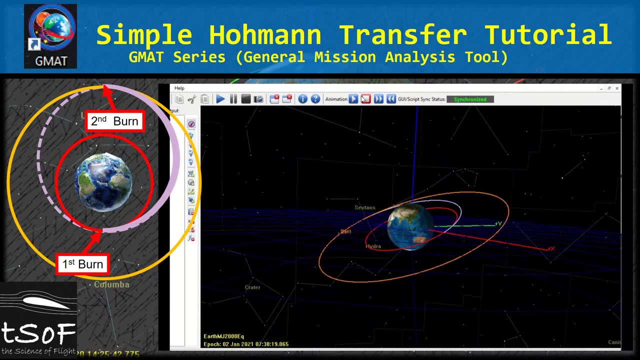 from one circular orbit about Earth into a different circular orbit about Earth. So we'll start out talking about what that Hohmann transfer is and what I'm talking about when I'm saying these different circular orbits and stuff, And then we'll get into the tutorial to show. 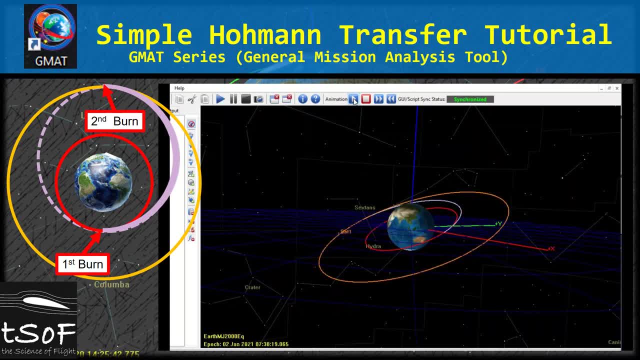 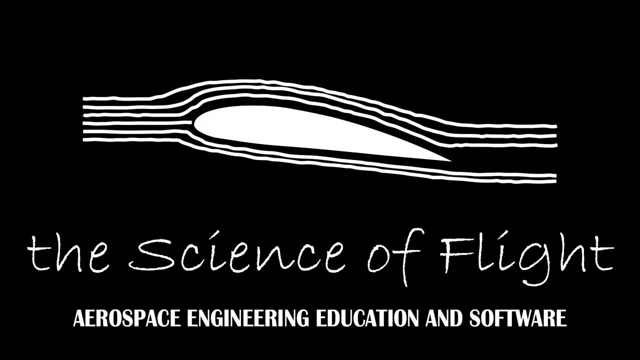 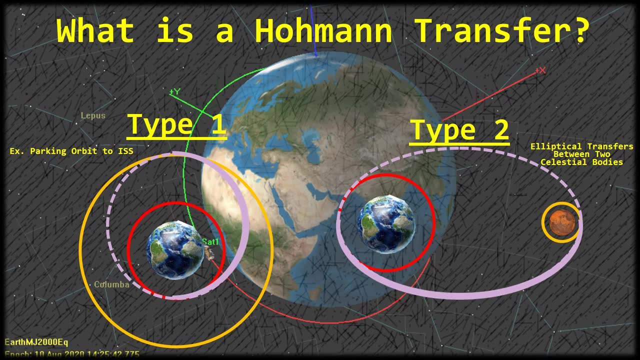 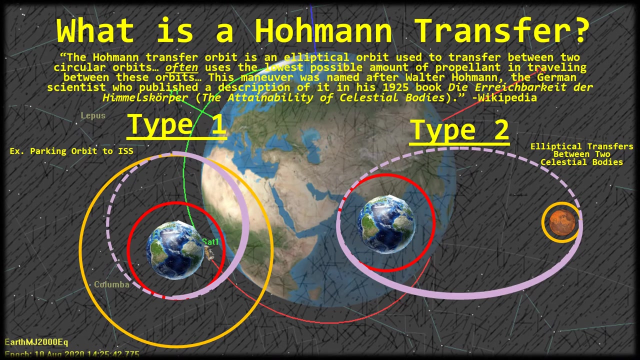 you how to set up this simple Hohmann transfer in GMAT. Let's get to it Now. before we begin the tutorial, let's take a quick second to review what a Hohmann transfer is. I got a definition off of Wikipedia. You know it's not always the best source. 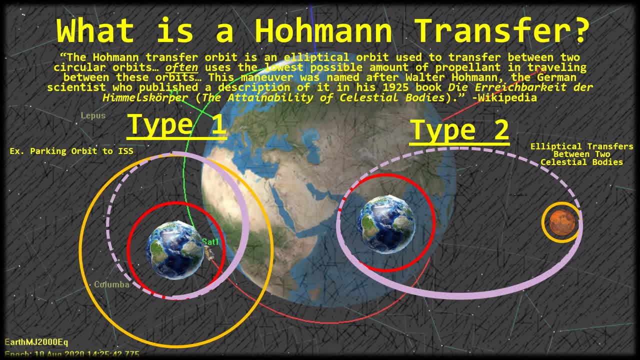 but it's got not too bad of a definition here So let's use it. It says that the Hohmann transfer orbit is an elliptical orbit used to transfer between two circular orbits. As you can see, here we've got the red circular orbit and the orange circular orbit. The Hohmann transfer would be the purple. 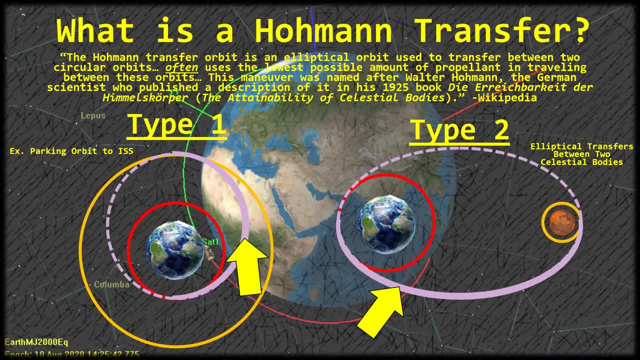 elliptical orbit. And then, going back to the definition, it says this often uses the lowest possible amount of propellant in traveling between these orbits. There is other orbits that sometimes use less propellant. So let's take a look at the Hohmann transfer. So let's take a look at the. 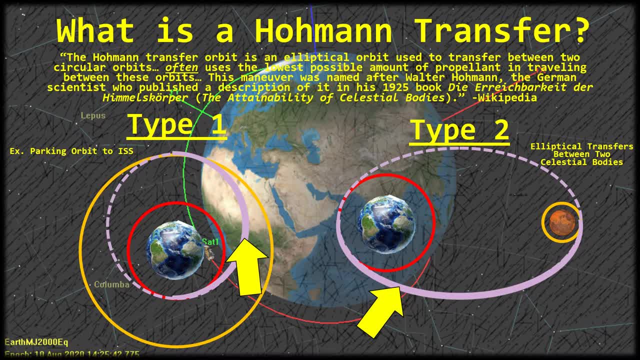 CES like the Bileptical Transfer Orbit, and you know we'll probably cover that in a future video. And of course, it's called a Hohmann transfer because it's named after Walter Hohmann. Now these transfer orbits are needed when we're trying to go from a starting orbit to a final. 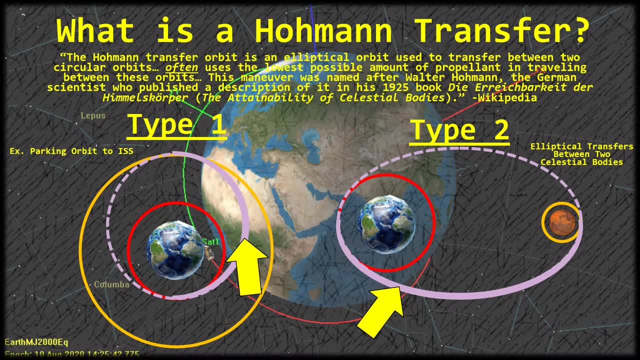 orbit and those orbits don't ever have any points in common, right? There's not a point where you could be on both orbits? If that were the case, then we wouldn't need a transfer orbit. We can just do a simple burn to go from one orbit to the next. 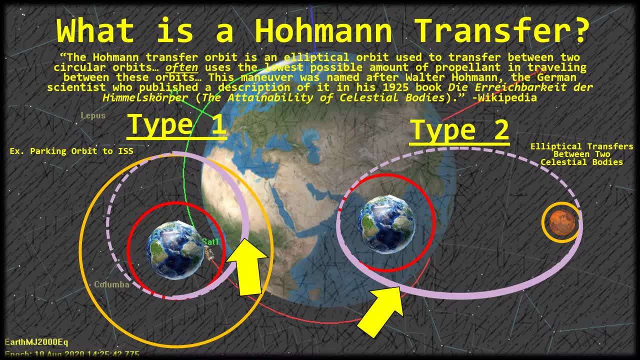 wall. we're at that common point. But since we're starting on one orbit, we're going to a different orbit. that don't touch right. They don't have any points in common. It means we're going to have to do a first burn from that starting orbit to get onto a transfer orbit And then, when that transfer, 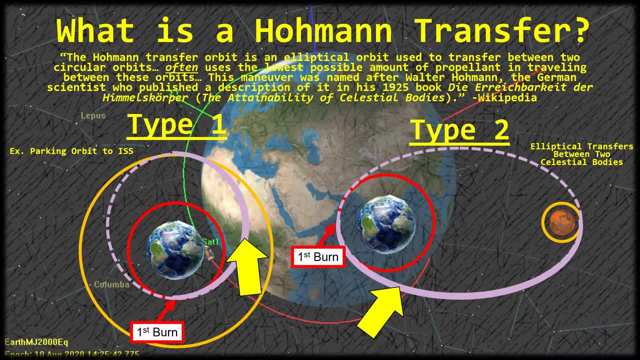 orbit comes into contact with the final orbit that we want to get to, we're going to have to do another burn to get off of the transfer orbit and to stay in that final orbit. And so this Hohmann transfer is a simple type of that, where we're going from one circular orbit to another circular 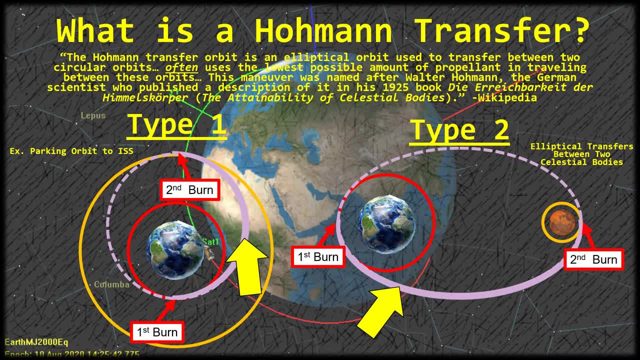 orbit using a Hohmann transfer orbit or this elliptical orbit. Now what does that mean? in the real world, That means usually one of two things. We could be going from one circular orbit to a different sized circular orbit around the same body, like you see here on the left. 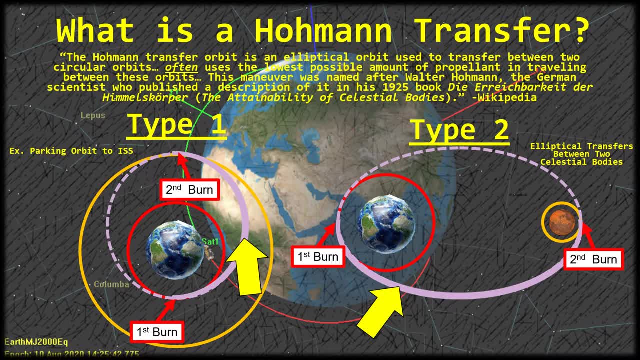 Some examples might be: you know, your launch vehicles put you up in a parking orbit, but you actually need to travel up to a higher orbit. Maybe you're going to the ISS, or maybe you're going up to a geosynchronous altitude, And so you've got to get up to a higher orbit. 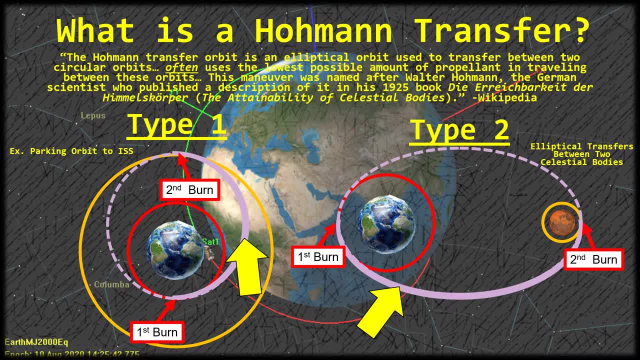 so that's one kind that you see here on the left And that's the kind that we're going to do in this video. Now there is another flavor of this particular transfer orbit. You could start with a circular orbit around one body and then use the Hohmann transfer to get to a circular 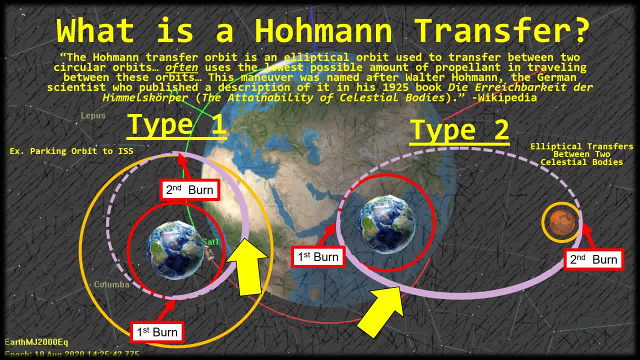 orbit around another body I've got pictured here on the right. the first orbit is that red one that circles the Earth, And then you might perform your first burn to get onto that transfer orbit that will eventually take you to Mars. So when you get there you're going to have to get. 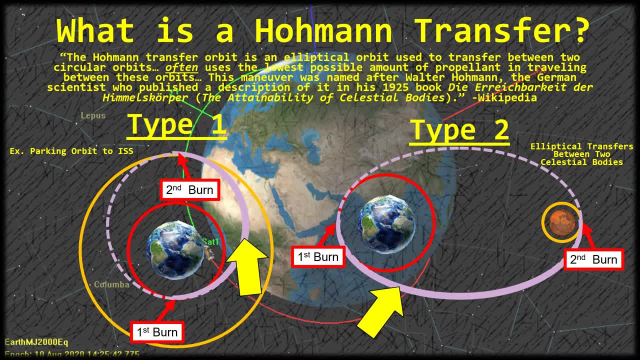 there you'd have to perform your second burn to go from the transfer orbit into that final orbit around Mars. Now this second type of problem is a little bit trickier, because it's not just a matter of geometry, it's also a matter of timing as well. If I perform this maneuver right, I start in my 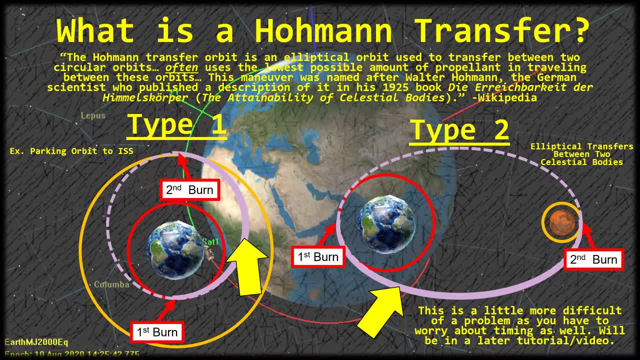 parking orbit. I perform my first burn and I'm in my transfer orbit and I get out to where my second burn is supposed to occur and I didn't time it right, so Mars isn't even there. then that second burn's not going to do anything, So I'm going to have to do a circular orbit and then I'm going to 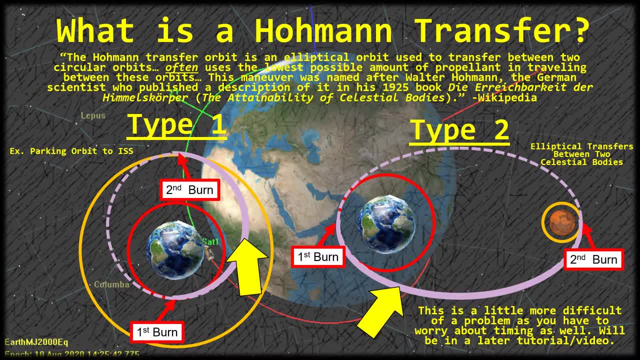 do anything right, It's not going to put me in a parking orbit above Mars because Mars isn't there. So with this type, we also have to worry about that timing, And you'll see what I mean in a future video- when we do one of those home and transfers. For the first step, let's go ahead. 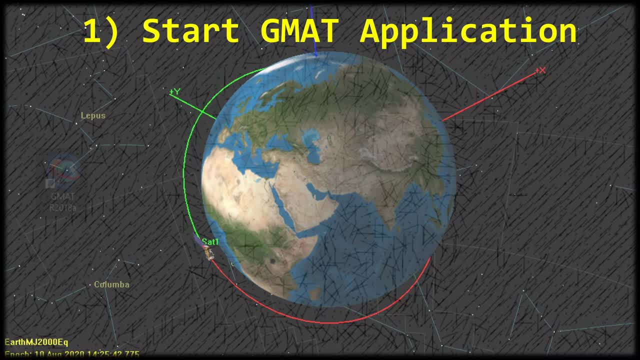 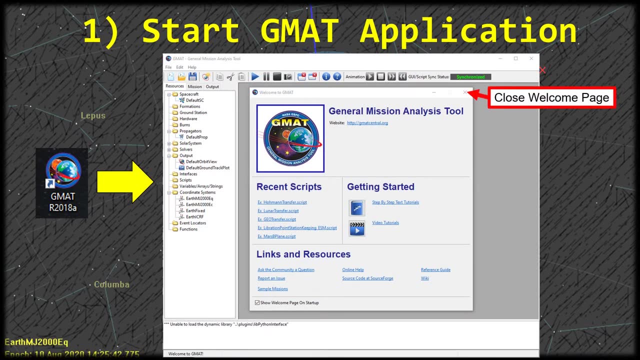 and start the GMAT application. So look for a shortcut like this: When you start it up, it's going to open up the welcome page. You can go ahead and click that x in the top right to close the welcome page. Next step: we're going to go ahead and start a new mission. 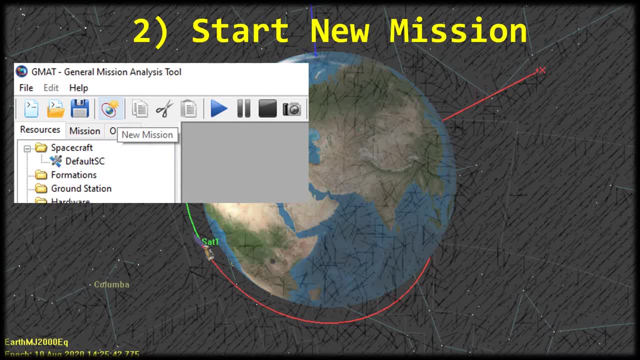 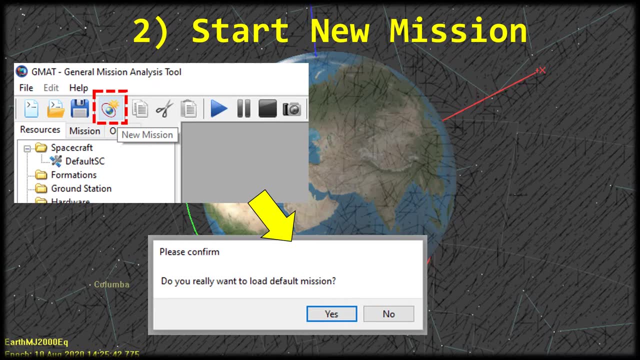 If you already had GMAT open and was working on something else, you can click this new mission button up on the toolbar. When you click that, it's going to give this pop-up that asks if you really want to load the default mission. Go ahead and click yes, And when you do that you'll see. 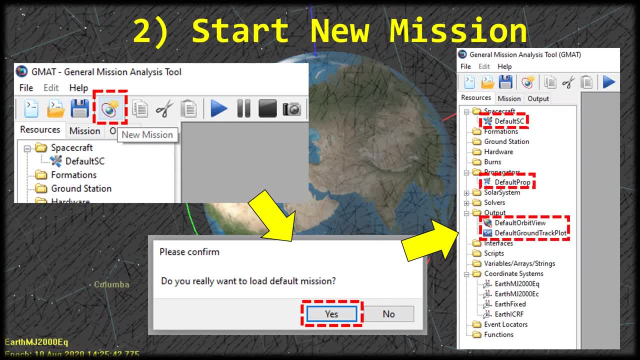 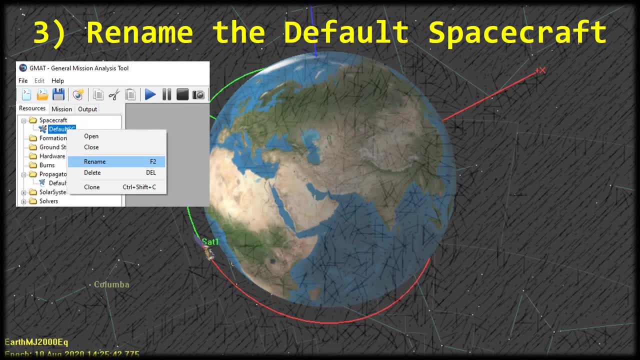 here on the left in the resources tab, all of the stuff turned into the default stuff. So you've got the default spacecraft, the default propagator, the default orbit view. Starting with the spacecraft, right click on default SC in the spacecraft folder. 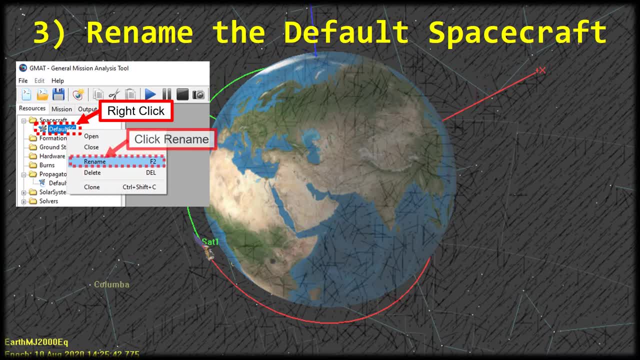 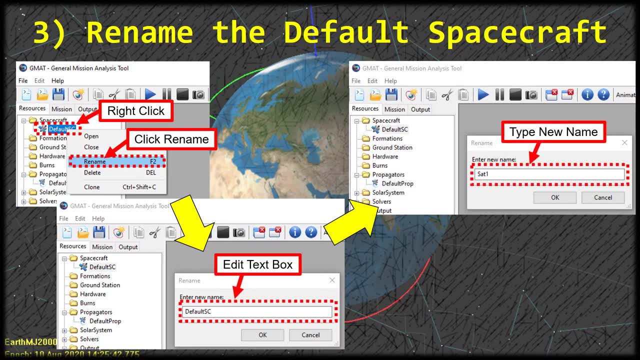 when you right click on that you'll see the menu pop up and we're going to click rename And that's going to open up this window here with an edit text box. We're going to type in the new name And so let's just go ahead and call that SAT1 for satellite one. So type that in the box. 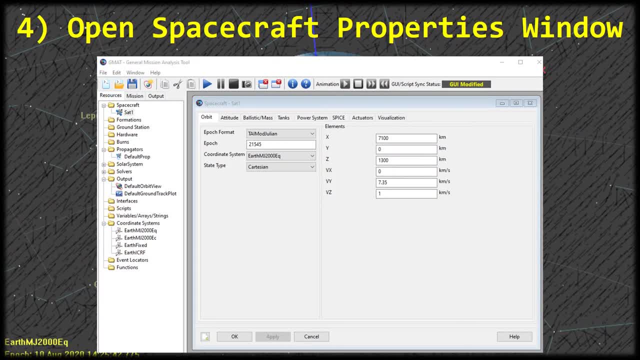 and click okay. Now that we renamed the satellite, let's go ahead and open up the spacecraft properties window. You can do that by double clicking on the object in the left project viewer. we renamed it SAT1.. So find SAT1 and double click on it, With the properties window open. 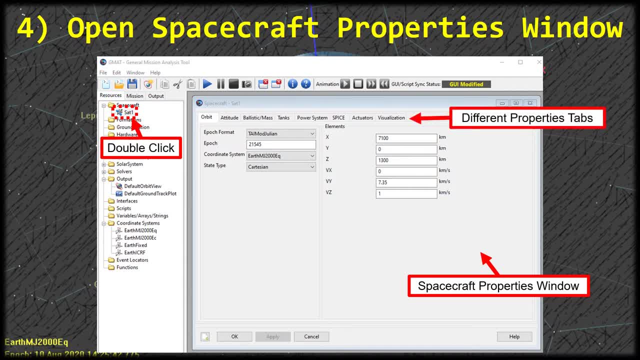 you'll notice that it has a bunch of tabs at the top. Each of those tabs have a group of different properties of the spacecraft. For this tutorial, we're going to just focus on a simple orbit, And so we're going to stay here on the orbit tab and adjust those parameters only In future videos. 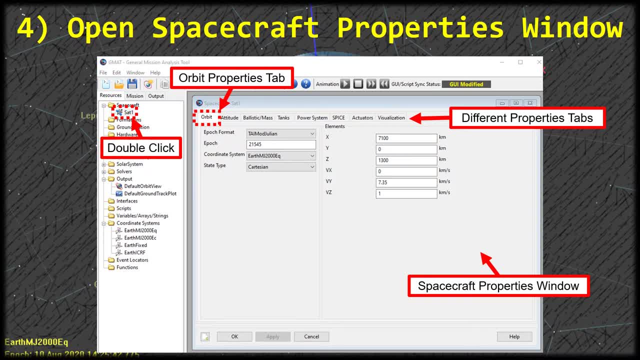 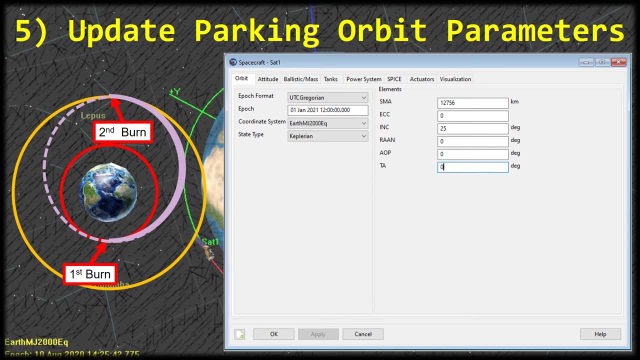 we'll cover some of the other tabs and properties in those tabs. So we're going to go ahead and update that. I'm just going to go ahead and update the orbit parameters. There's a couple of stuff. If you go to orbit, the first thing here is the coming orbit parameters And then, if you go, 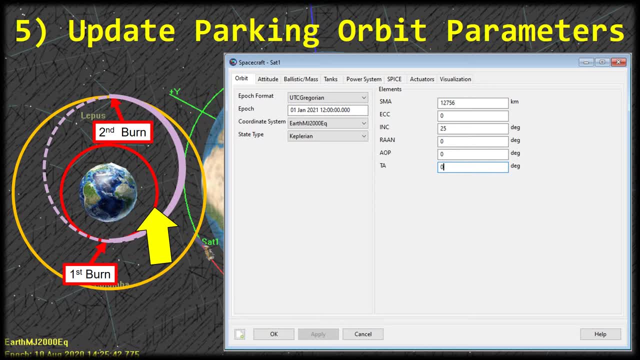 to get to the progress tab, let's go ahead and go ahead and update the orbit parameters. So here on the left, that would be the red orbit. This is the initial orbit that we're starting from. This might be the orbit you would get to after your launch vehicle takes you up to orbit, Or 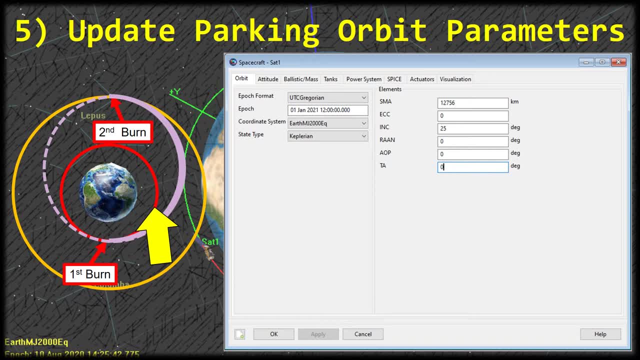 if you're a satellite and your orbit has decayed and you're about perform a couple of maneuvers to get back up to the orbit you're supposed to be in, this red orbit might be your starting point as well for this particular mission sequence. So the first things we want to do, 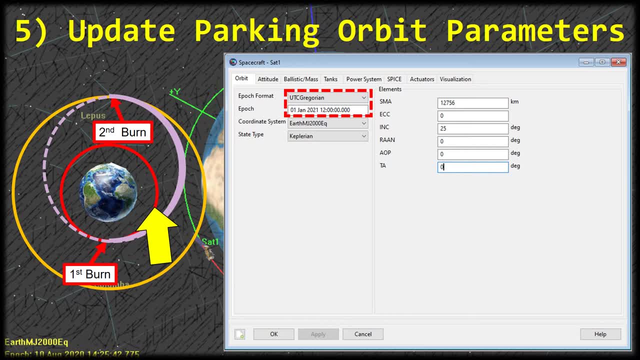 change that to UTC Gregorian And I just went and put January 1st of this year just for the heck of it- It doesn't really matter that much for what we're doing right now- And then going down to state type, I changed that to Keplerian And so that changes the elements here on the right And 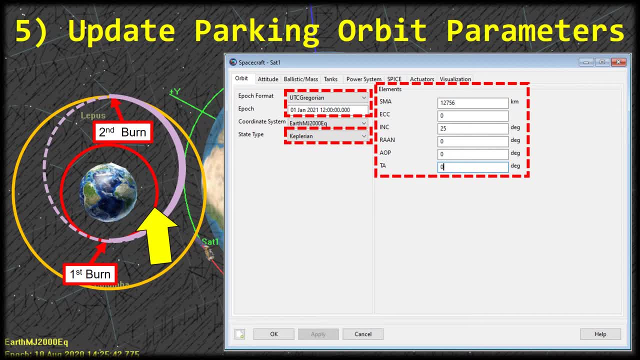 I can go ahead and update those parameters. I'm going to choose a semi-major axis of, let's see, 12,756 kilometers, That's about twice the radius of the earth- And then, of course, the other important thing is putting an eccentricity of zero. That's going to make 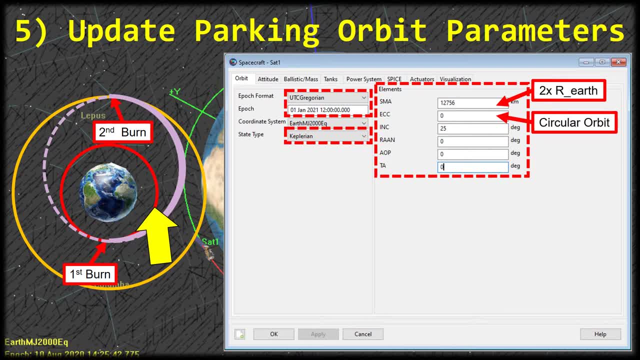 our orbit circular. And then I went ahead and put an inclination of 25 degrees, just for the heck of it. You could have left that at zero, or the rest of them at zero too. Those don't really matter so much. The parking orbit, the transfer orbit, the final orbit, they're all in the same. 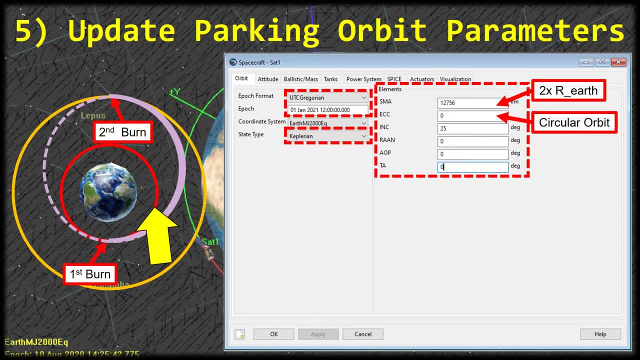 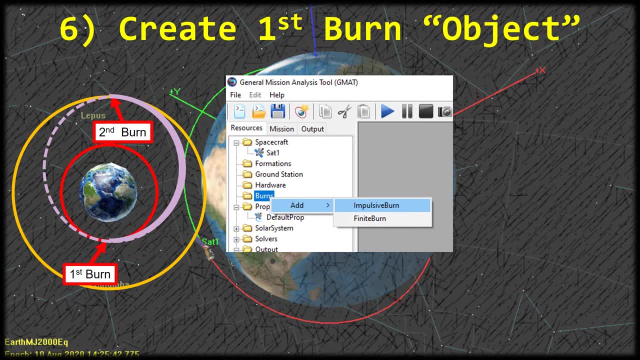 plane, So we don't have to worry so much about some of these values. So go ahead and update those values and click OK. when you're done, The next thing we're going to do is we're going to add the first burn maneuver. 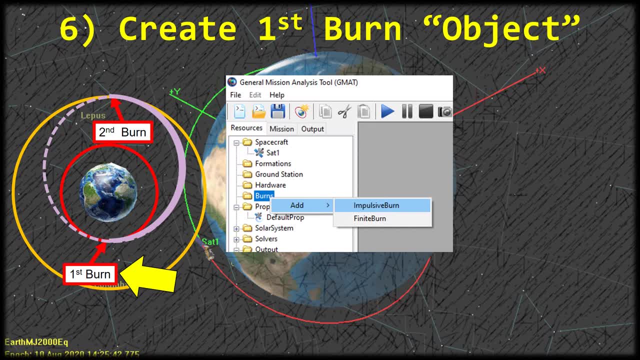 This would take place when we're trying to go from the red parking orbit to the purplish transfer orbit that you see here on the left. To do that, right-click on the burns folder and then find add and click impulsive burn. The difference between an impulsive burn and a finite burn is that an 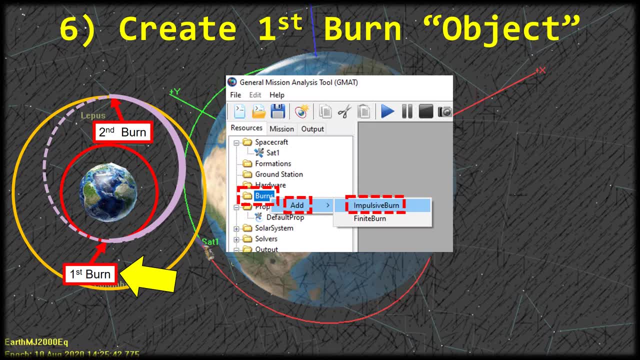 impulsive burn is just going to give you the entire delta V instantaneously. That has the effect of when the burn occurs, of changing from the red parking orbit to the purple transfer orbit instantly, versus a finite burn where I don't know, for example. 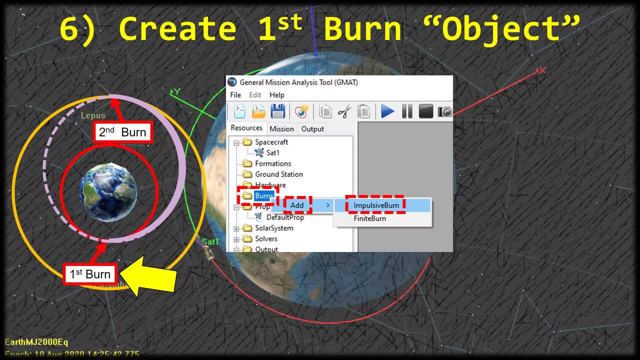 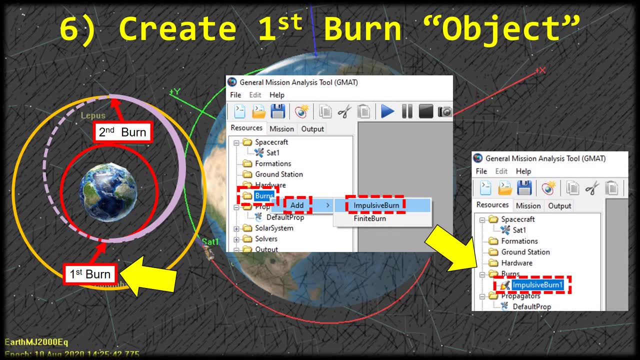 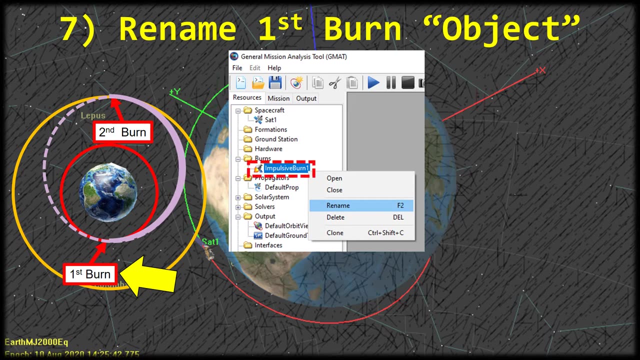 you might start the burn and it takes 30 seconds to achieve the entire delta V. So click impulsive burn and you'll see it show up in the left tree. Let's go ahead and rename this burn object. If you right-click where it says impulsive burn in the tree, it will pop up this context menu and 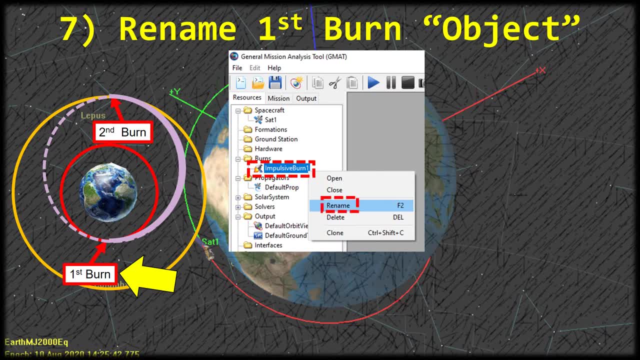 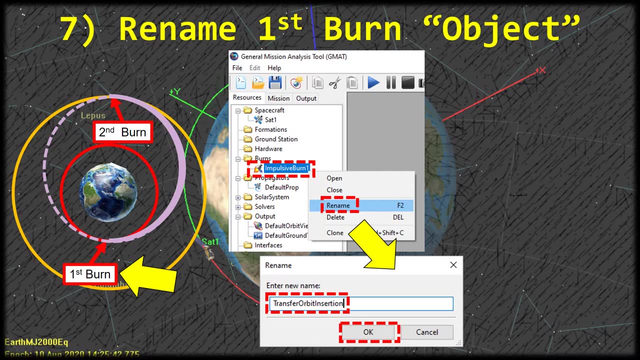 you can find the item that says rename. Go ahead and click that. That will open up this window here where you can type in the new name you want to call it and click okay, For this example, I'm just going to call this the transfer orbit insertion. This is where 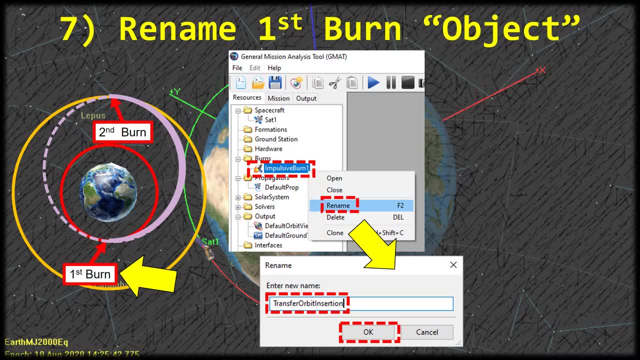 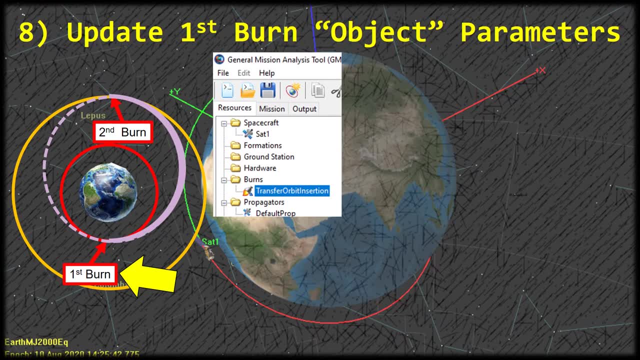 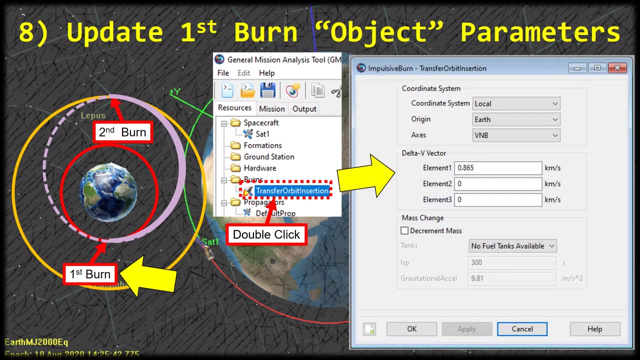 we're inserting the spacecraft into the transfer orbit. So when you click okay, you'll see that it has the new name there in the resources tab on the left. Now let's go ahead and double-click on that transfer orbit insertion burn in the left resources column to open up the menu or the 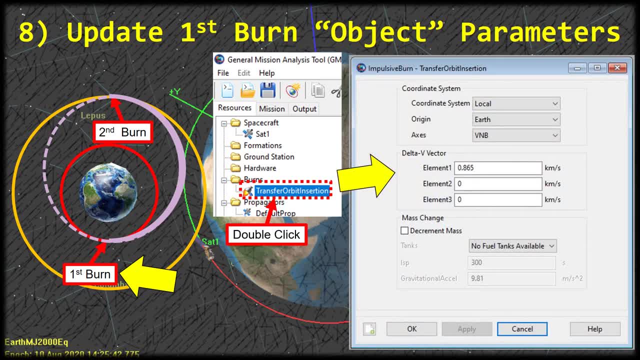 window us to adjust its properties And when that opens, we're gonna go ahead and add the delta V that we want right here in the first box at 0.865 kilometers per second. As you can see above here, that's going to be in the V and B coordinate. 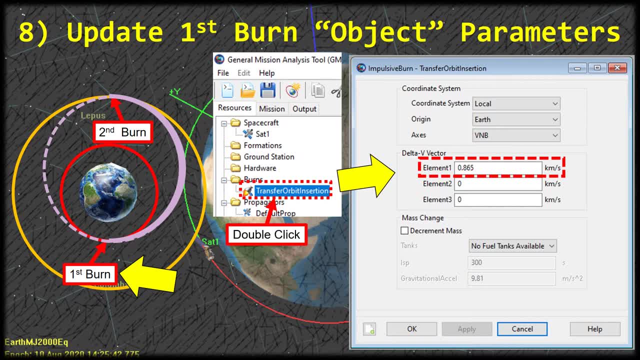 system, And so this first box corresponds to the V in V and B. That V in the V and B is gonna be what you see here on the left, But for now let's just go ahead and put in the value and click OK. Alright, let's go ahead and create the second. 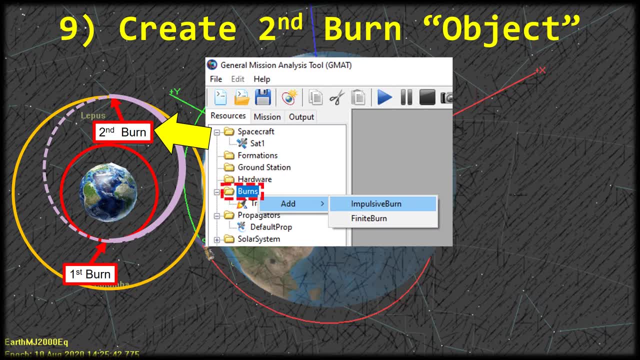 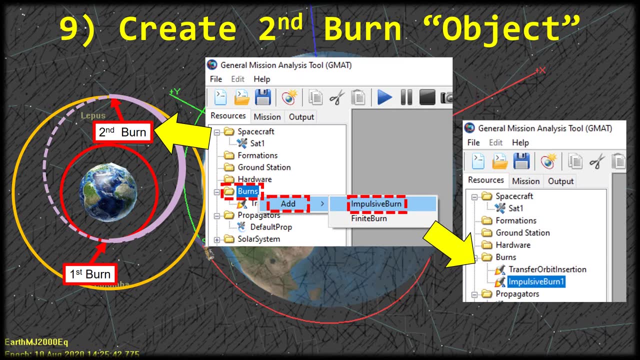 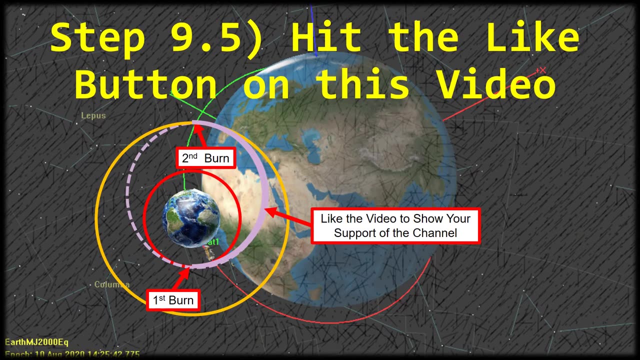 burn object. So again, right click on the burns folder, go to add and click impulsive burn. When you do that, you'll see it appear in the resources tab on the left right here, named impulsive burn 1.. Now the next step- step 9.5, is to hit. 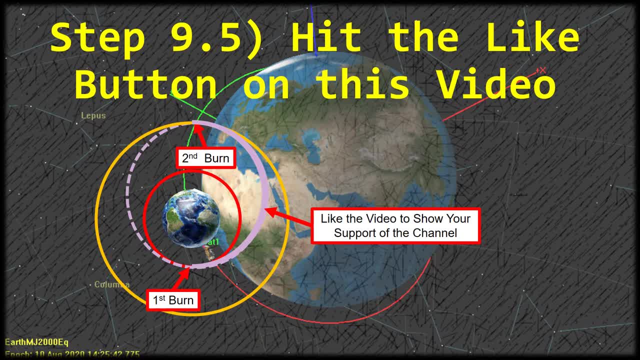 the like button on this video. Now, this is a very, very, very important step in this tutorial. Obviously, if you're not familiar with this tutorial, you can do this for yourself. It's not going to work without it. Go ahead and hit that like button Again. we're gonna go ahead and rename this object that we just 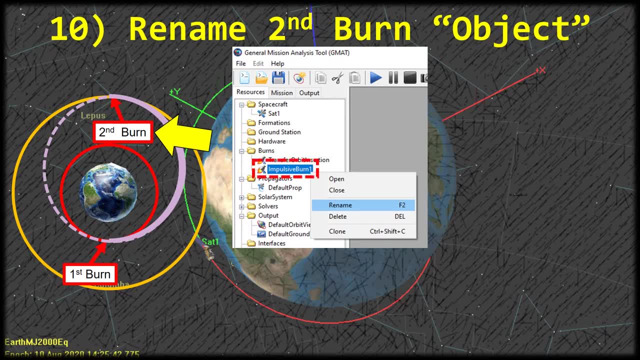 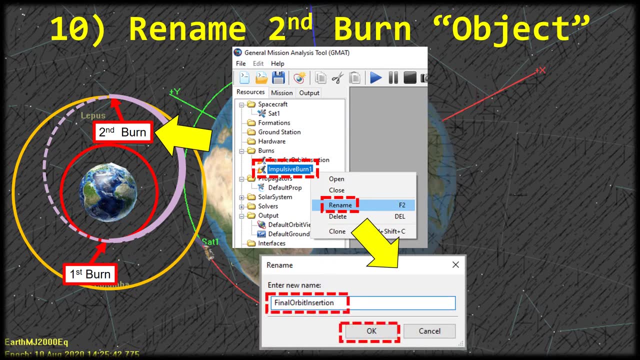 created. So right click where it says impulsive burn and in the menu that pops up click rename And that window that pops up type in final orbit insertion and click OK. This is gonna be the second burn that we used to go from the transfer orbit into the final orbit, so that's why we call it final orbit. 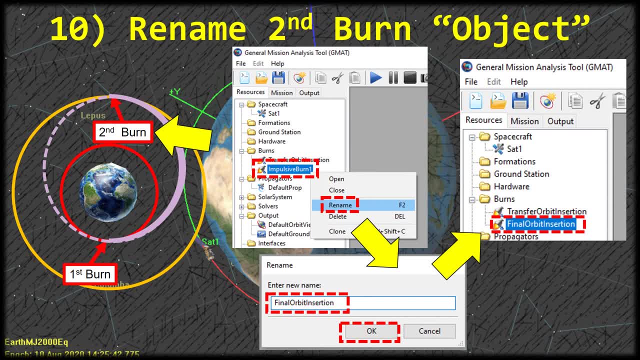 insertion: After you type in that name, click OK and you'll see it there on the left in the resources tab. Go ahead and hit that like button And then you're gonna hit the next button. Go ahead and double click on that final orbit insertion to pull up. 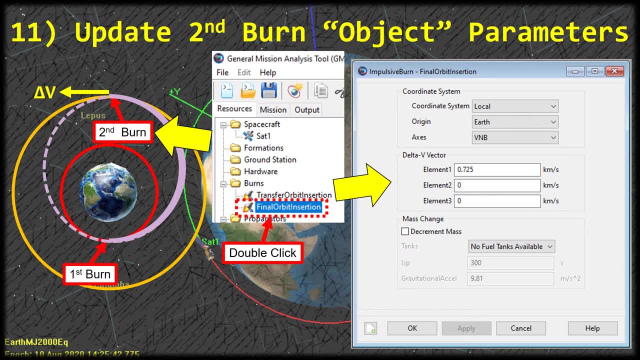 its properties window. When that appears, we're gonna go ahead and give it a delta V of 0.725 kilometers per second And, as you can see up above, we're in the V and B coordinate system, So we're giving this a delta V of 0.725 in that V of the V and B. 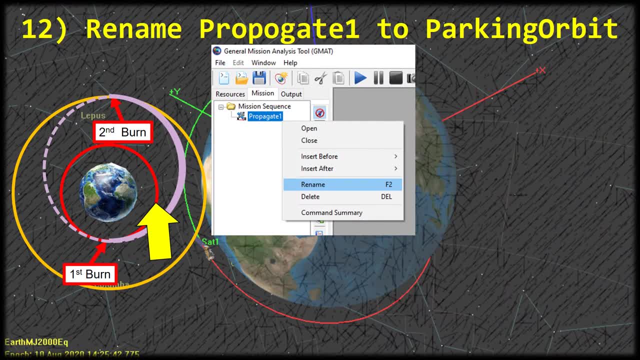 coordinate system. Go ahead and click OK, Alright, so we've gone ahead and created all the objects that we need in our mission. So we're gonna go ahead and create our mission. So we're gonna go ahead and click over to the mission tab and we're gonna start building out our mission. 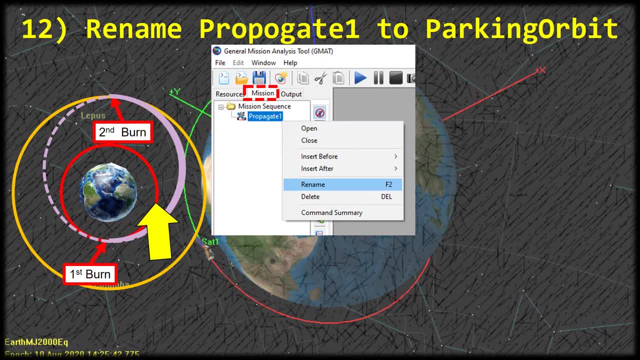 sequence Right. what are the order of the events that is going to occur with the objects we created? You'll see that it already has the default propagate one in it. Let's go ahead and rename that to parking orbit. So right click on it and 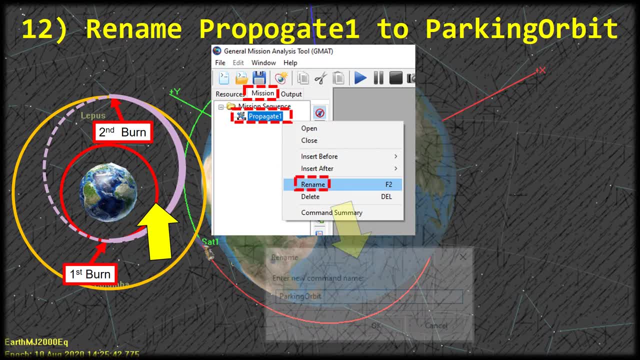 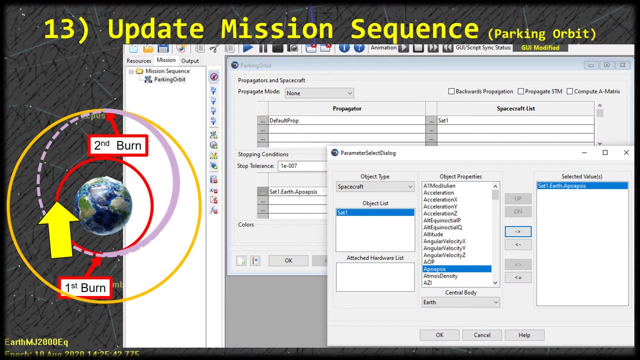 the menu that pops up, click rename. In that window that pops up, type parking orbit and click OK And then you'll see that the name changed in the mission tab on the left. Let's go ahead and double click on that parking orbit event in the mission sequence And in the window that pops up. 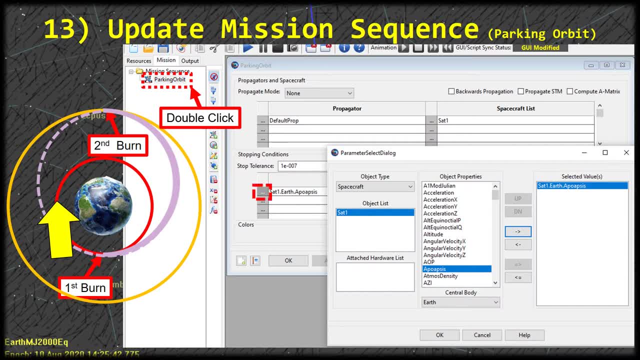 we're gonna double click on these three little dots on the left to change the default stopping condition to be what we want it to be. So in this list, go and find apoapsis Just as a quick double check. make sure that that central body. 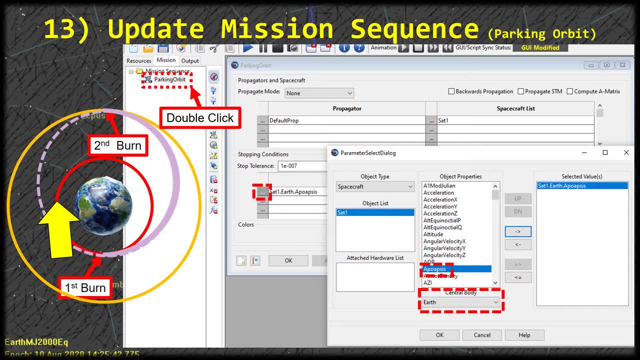 says earth. We don't want to stop this at the apoapsis around I don't know the Sun which could be in a different part of our orbit, So make sure that says earth. click the arrow to move it over to the right as a selected value. 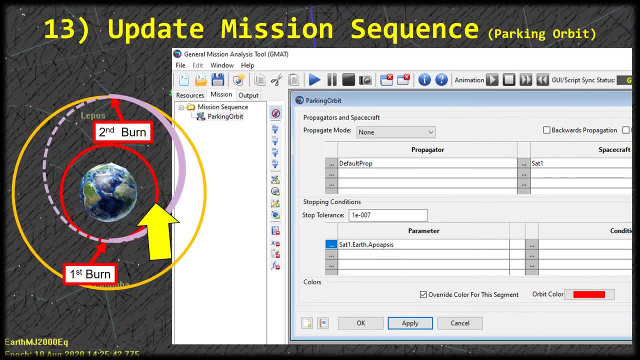 you. When you've done that, go ahead and click okay. As you can see here in this propagate window, the stopping parameter has changed to be sat1- earth apoapsis, which is what we want. Now I'm going to go ahead and click this check mark to override the color for that segment and I'm 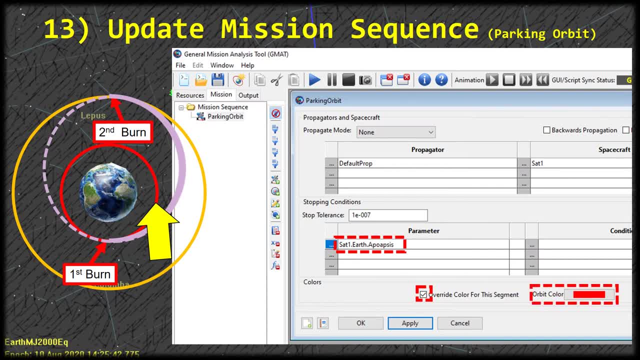 going to make the color red to match this drawing that I have here on the left. You don't need to do that if you don't want to. So after I do that, I'm going to go ahead and click okay to save the changes to this first event. right, this propagation event. So this first event took 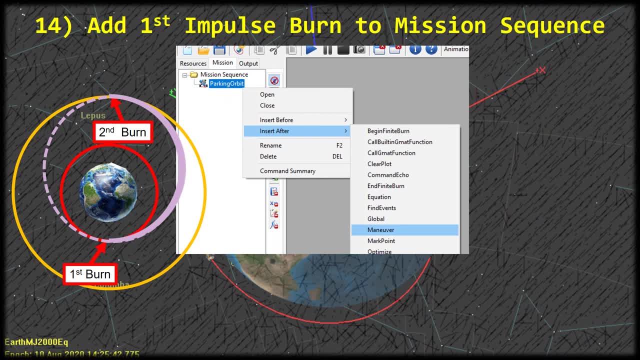 care of moving the aircraft on that red orbit right, propagating it on that orbit. Now it's going to stop at apoapsis, which is where I want to start the home and transfer, And so what I'm going to want to do is that, after that parking orbit, I'm going to want to insert this first: 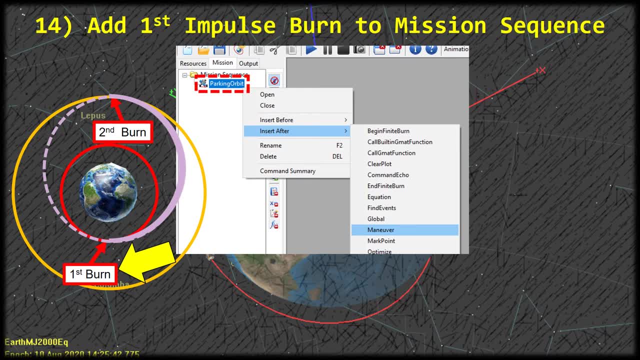 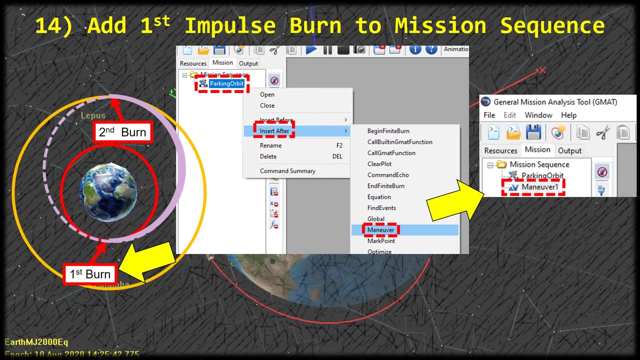 burn. To do that I right click on parking orbit, go to insert after, and then I find maneuver and I click on it And then you'll see that it will add this delta v maneuver in the mission sequence. It's called maneuver one. So go ahead and double click to open up that maneuver and 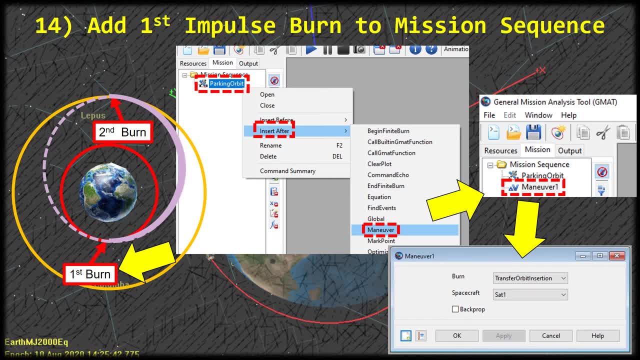 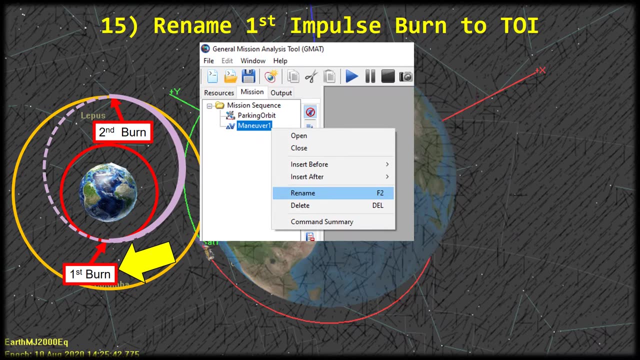 you'll see that you have the option of choosing which burn that that maneuver is. Since this is the first burn that's going to insert us in our transfer orbit, I want to make sure that I have the transfer orbit insertion burn selected in that burn and click okay. So let's go ahead. 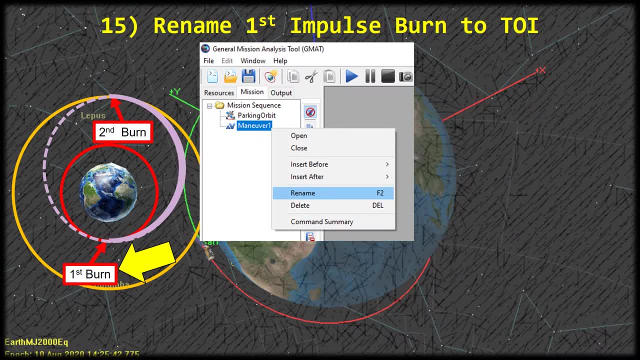 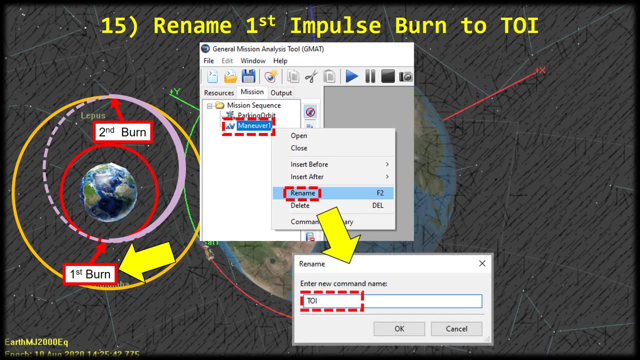 and rename this first impulse burn to TOI, That stands for transfer orbit insertion. On that maneuver, one object. go ahead and right click in the menu that appears, find rename and click on it. And then in the window that appears after that, go ahead and type in TOI and click okay. 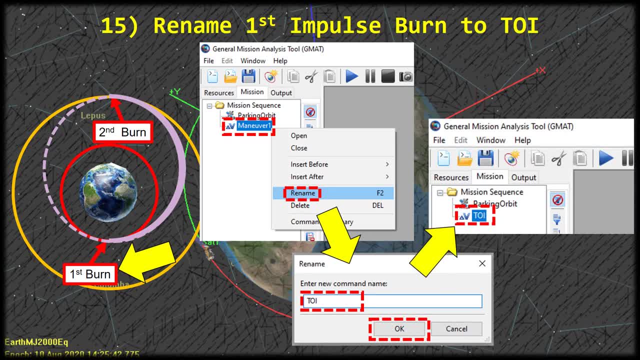 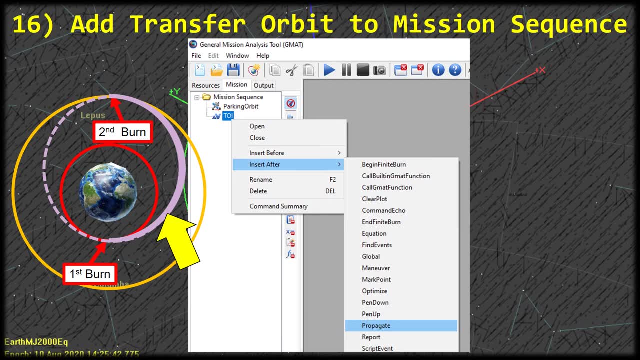 And you'll see that the name changes here on the mission tab on the left. Now, as I talked about before, the burn is an impulsive burn and so it adds all of the delta v instantaneously, And so it has the effect, essentially, of changing from one orbit to the. 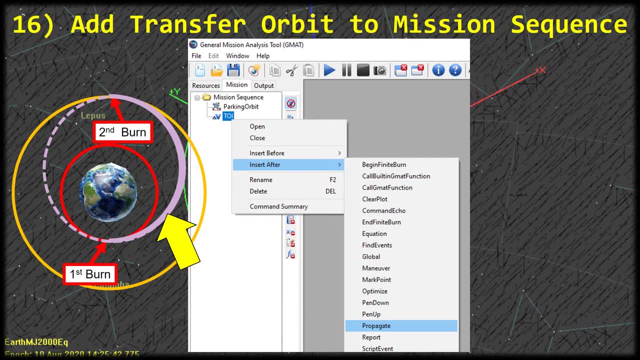 next instantly. You don't have to wait through a finite burn where it takes so much time to actually get all the delta v. Now, if you look at the mission sequence and if we left it just right here, essentially what we're doing is we're orbiting on that parking orbit and then we do. 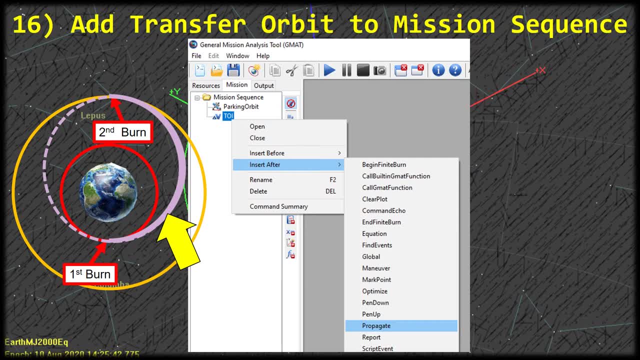 the burn to change orbits, but we don't do anything. So if you went ahead and went play on the simulation now, you'd only see the red orbit. What we need to do is that now that we're on the transfer orbit, we're going to go ahead and change the orbit, And so we're going to go ahead and. 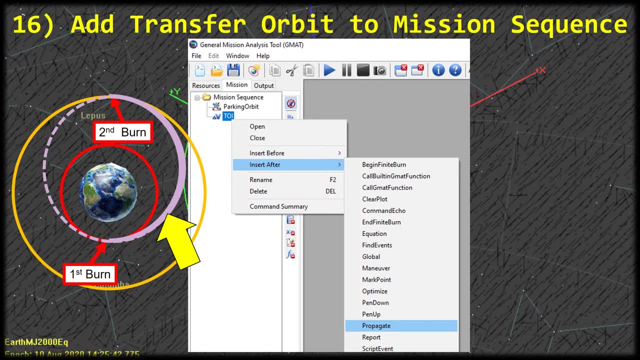 transfer orbit. after this maneuver We need to actually propagate the spacecraft on this transfer orbit for a certain amount of time. So in the mission sequence on the left, go ahead and right click on the TOI burn. In the menu that appears, click insert after and then we're going. 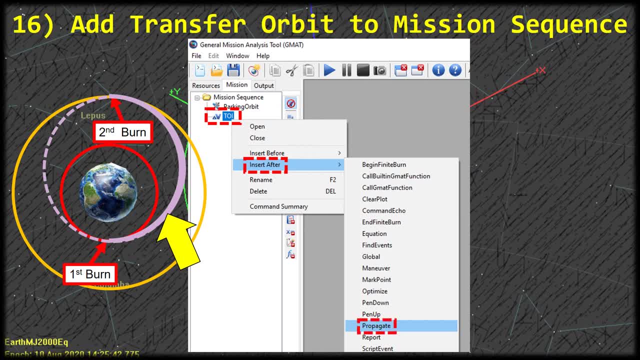 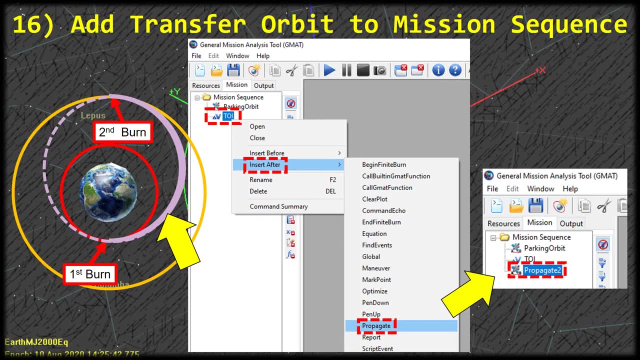 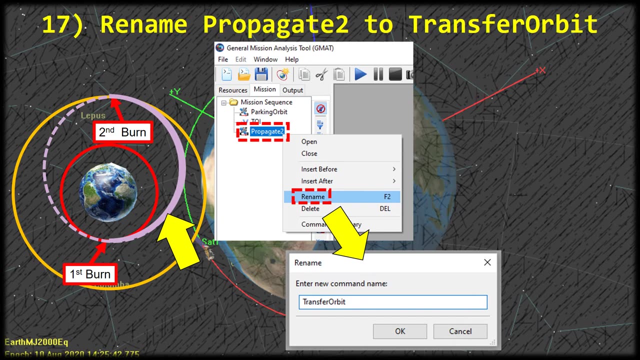 to go in the next menu that appears and find propagate and click on it And you'll see it appear here in the mission sequence. on the left It's named propagate 2.. Now let's go ahead and rename it from propagate 2.. So right click on it, click rename, and the window that appears type in. 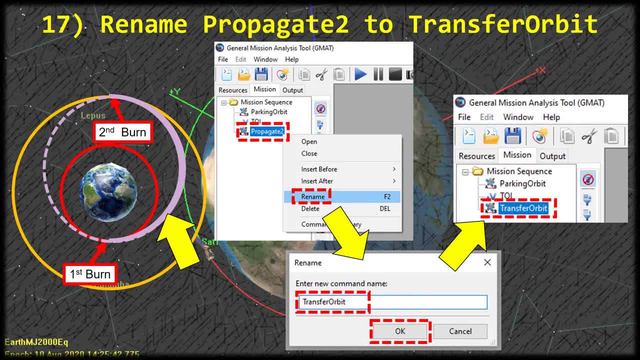 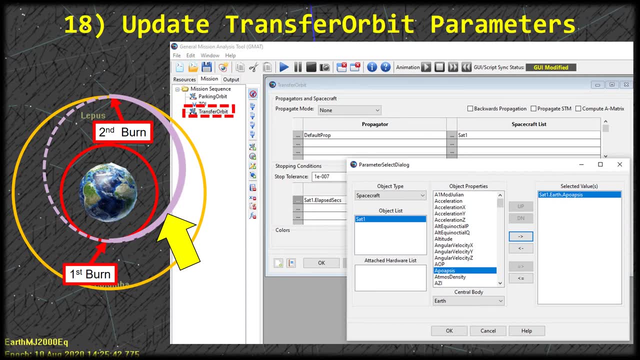 transfer orbit and click okay, And then you'll see there on the mission sequence on the left that the name has changed to transfer orbit. So go ahead and double click on that transfer orbit to open the propagation properties window. and we're going to go ahead and change the stopping condition by 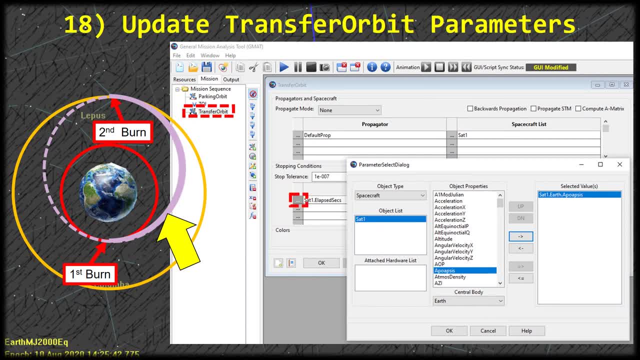 clicking on these three circles on the left, and we're going to change it from elapsed seconds. We want to propagate this spacecraft to the apoapsis point of the transfer orbit. That's the idea behind this Hohmann transfer is that we start. 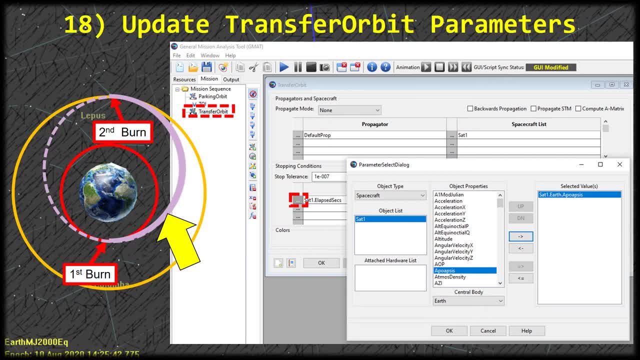 at the periapsis of the orbit and we size it so that we get to the apoapsis of the transfer orbit when we're at that point where we want to switch to the final orbit. So find apoapsis in the list. 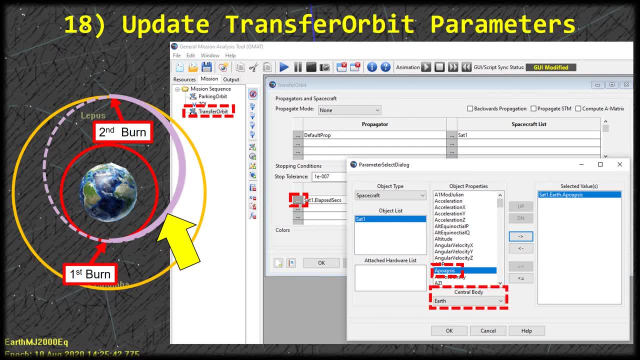 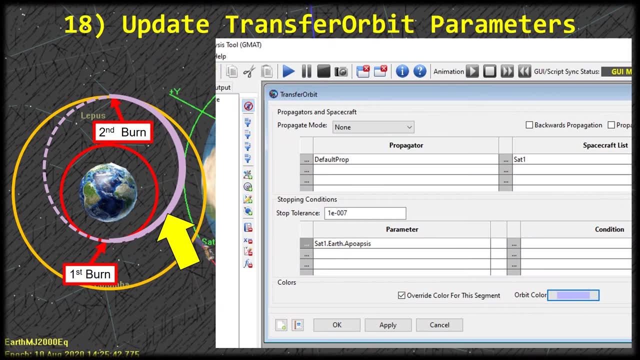 and make sure the central body of course is earth. Don't forget to click the arrow to actually change the selected value there on the right column and then, when you do that, click okay. You'll see that the parameter changed to apoapsis. Now I'm going to go ahead and do another step that you don't have. 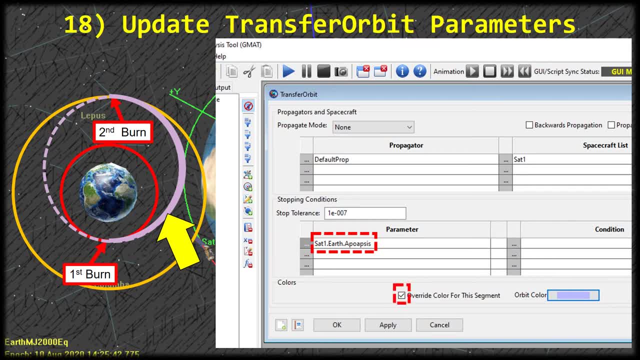 to do? I'm going to go ahead and click this checkbox here to override the color for the segment and then I'm going to search for this light purplish or pinkish, whatever color that is, so that when I'm on this transfer orbit you can see that it's a similar color. 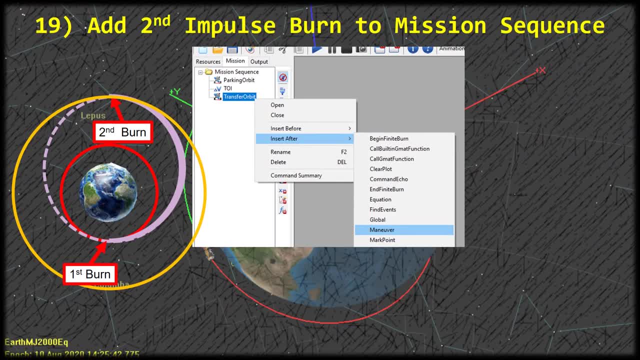 And then, when I'm done with that, I'll go ahead and click. okay, All right, so in the mission sequence we went ahead and reached the apoapsis of the transfer orbit, and so now it's time to perform the transfer orbit, So I'm going to go ahead and click okay. 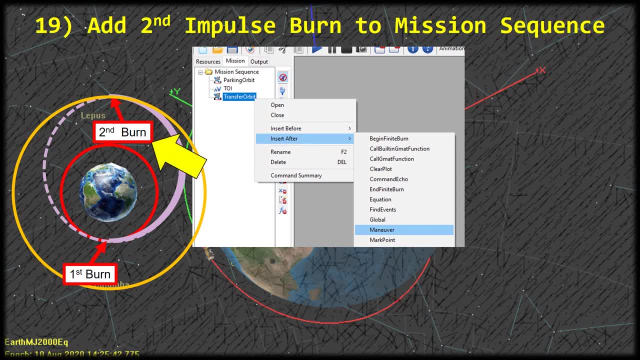 That second burn to insert ourselves into the final orbit, and so that means that we're going to have to right click on this transfer orbit, hit insert. after, In the menu that appears, we're going to click on maneuver and you'll see that that maneuver is added to the mission. 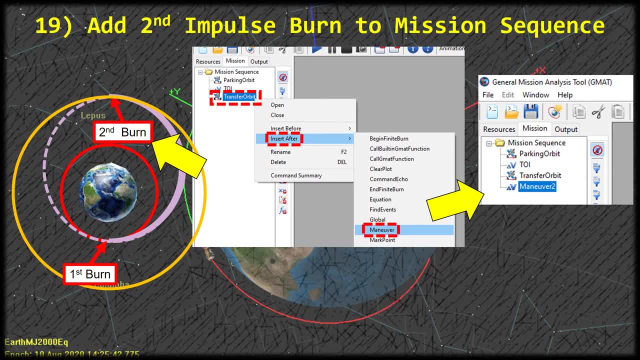 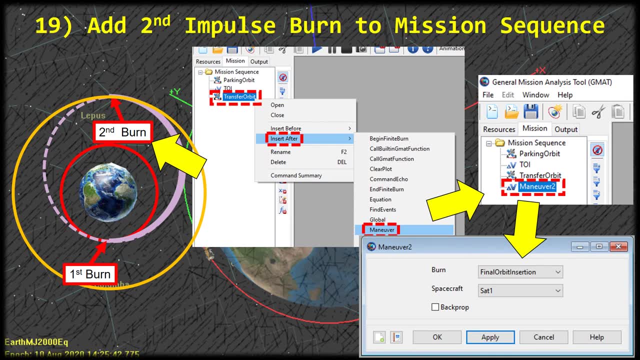 sequence. On the left it's called maneuver two. Let's go ahead and double click on that to open it up and since this is the burn that we want to insert ourselves into the final orbit, we're going to make sure that the burn in the drop down box says final orbit insertion. 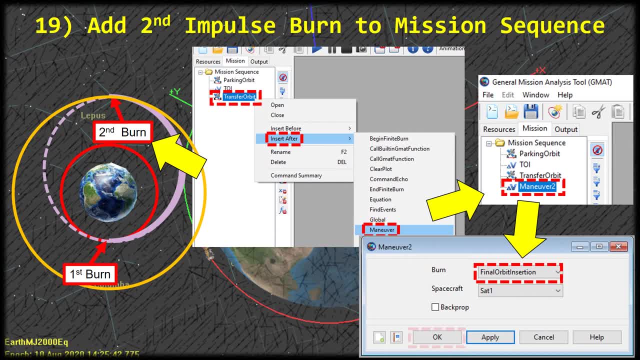 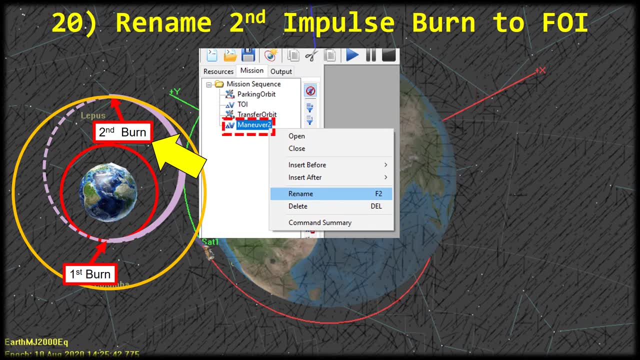 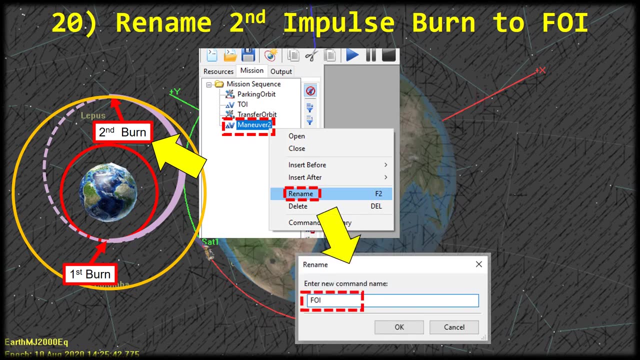 so go ahead and find that in the list, select it and click okay, Let's go ahead and just rename this burn. So right click on maneuver two and in the menu that appears find rename and click on it, and then in the window that appears after that, type in FOI for final orbit insertion. 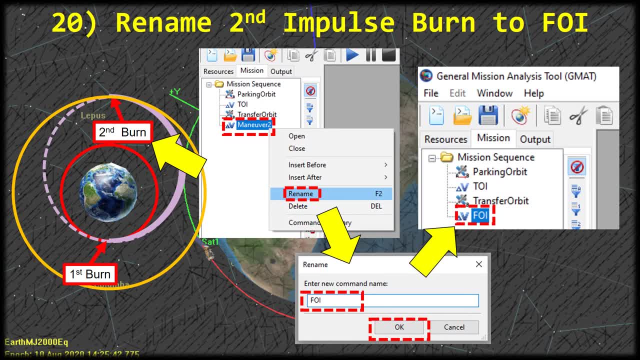 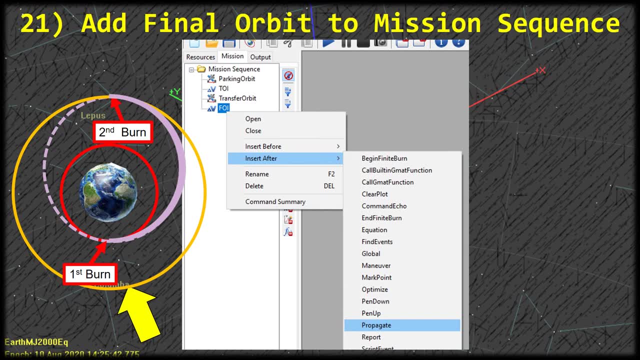 and click okay, and then you'll see that it changed the name here in the mission sequence. Okay. so where are we right now? We just finished the transfer orbit. We're at apoapsis of the transfer orbit. We can now do the final orbit insertion burn. Since this is an impulsive burn, that means we 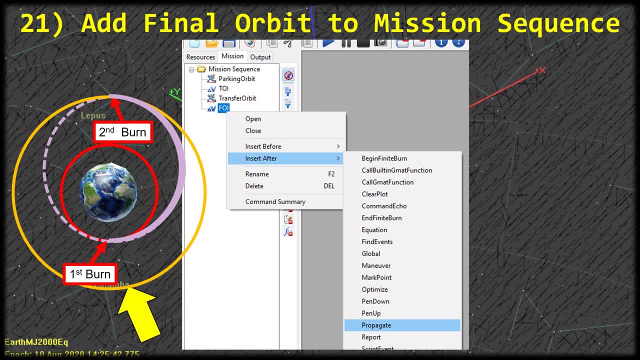 just instantaneously changed from the transfer orbit into this orange final orbit. Now if I stopped here and ran the simulation and showed it to you, you would see the red parking orbit, then you would see this purplish transfer orbit, but you wouldn't see this final orbit at all. 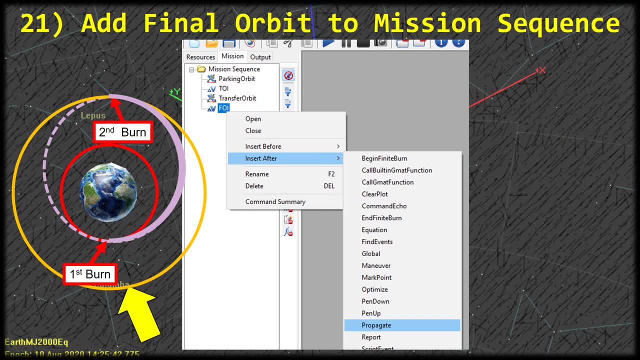 and that's because now that we're on the final orbit, we have to actually propagate the spacecraft on that orbit for an amount of time to be able to see it show up. So let's go ahead and do that. Right click on FOI and in the menu that appears, select Insert After, And then in the menu that, 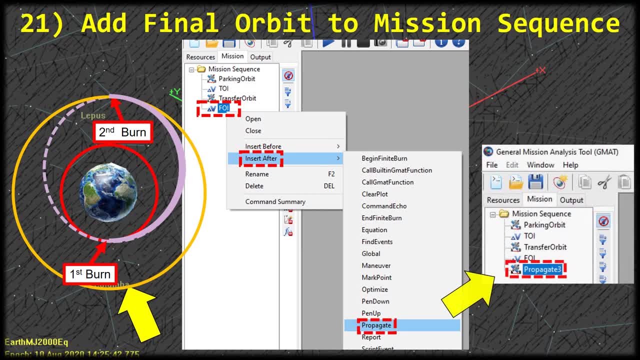 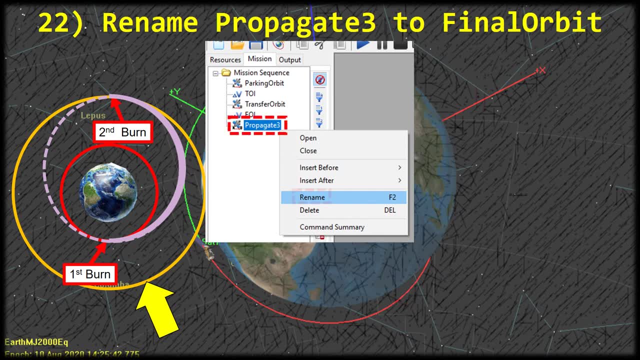 appears after that, select Propagate And you'll see it appear there in the mission sequence. Let's go ahead and rename this Propagate 3.. So right click on it and click Rename. In the window that appears, type in Final Orbit and click OK. And then there in the mission sequence tab on the 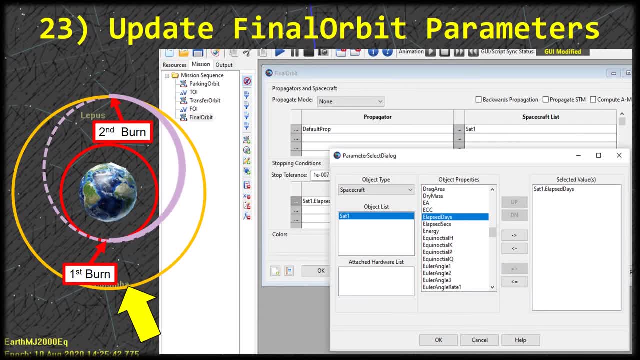 left, you'll see that the name has changed. All right, let's go ahead and update the Final Orbit parameters. So double click on the Final Orbit in the mission sequence on the left and you'll see the parameter window pop up. Now we're going to change the stopping condition by clicking the. 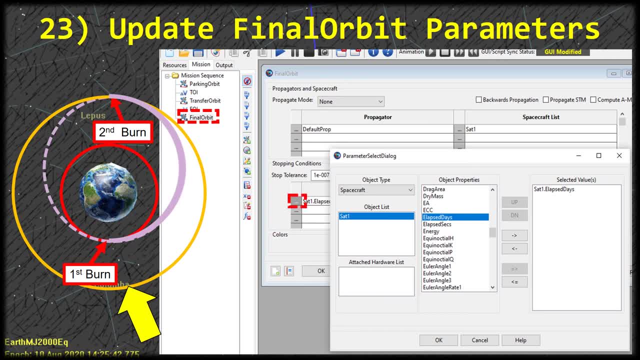 three buttons here on the left. I'm just going to go ahead and change it to be Elapsed Days, just because it's going to be pretty easy to just make it rotate for, I don't know, half a day or a day, just to get it to go around its orbit at least once, so that we can see it. 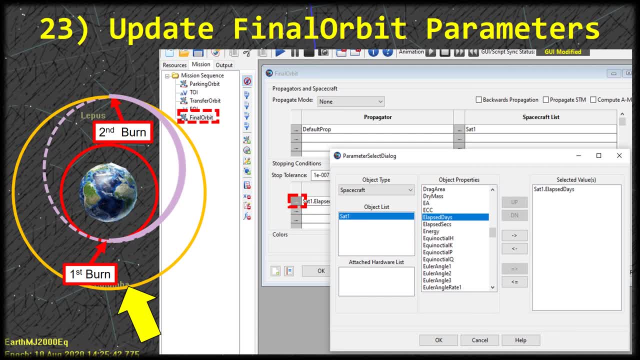 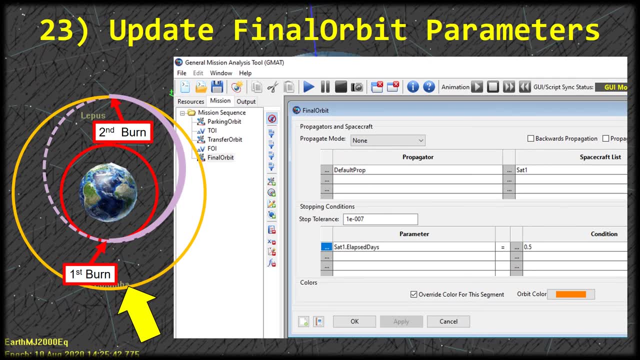 Doesn't really matter where it ends up. So go ahead and find in the list Elapsed Days and click the right arrow so that it becomes the selected value and click OK. You'll see that after I've done that, that the stopping parameter has changed to Elapsed Days, Since this requires. 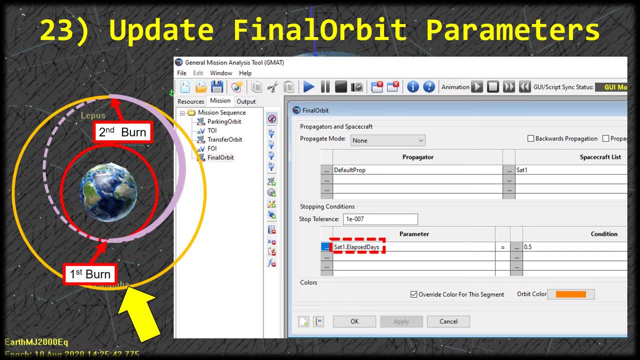 some additional input here. on the right, I'm going to give it a condition of 0.5. So this is going to propagate the spacecraft on this final orbit until the Elapsed Days has reached 0.5. Which should be enough for a complete orbit. Now I'm also going to go ahead and override the color. 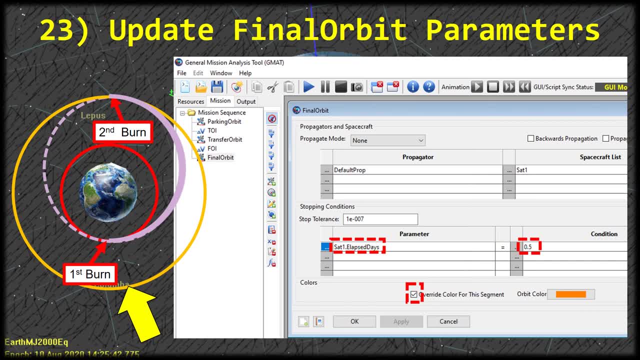 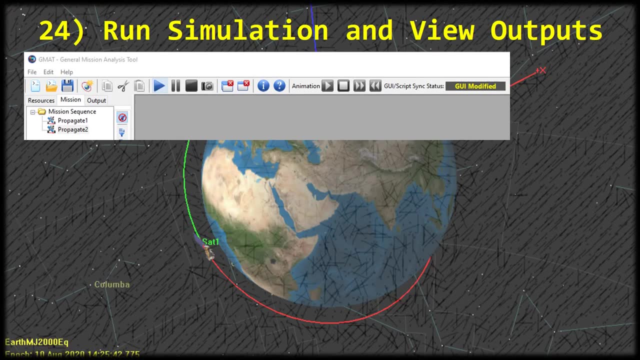 for this segment as well, by checking this box here on the left and then clicking on this color here on the right and finding the color I want. And so when I've done that, I'm going to go ahead and click OK to save the changes to this final orbit parameters. All right, we're done making changes. 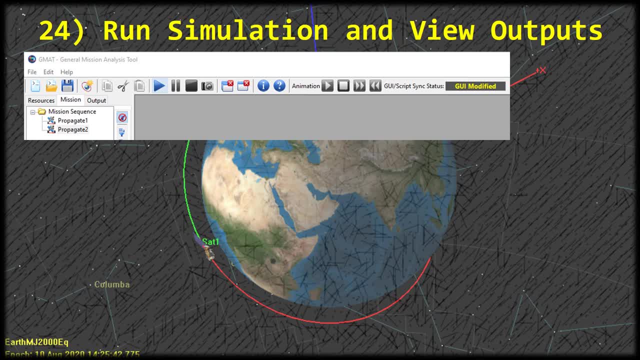 and updating both the objects and the events that we want to occur. And so now comes the point where we can actually run our project to simulate the mission sequence. So to run the simulation, you have the buttons here in the toolbar. We've got the play button, There's the pause button and stop. 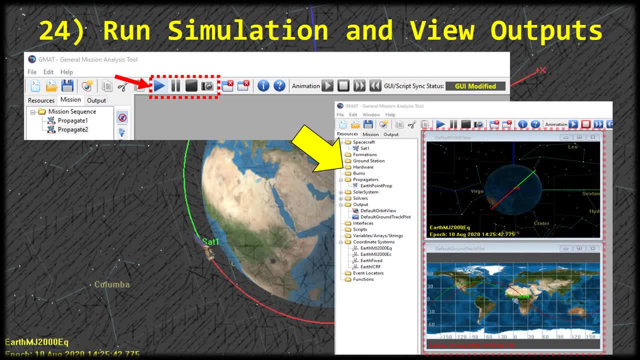 button And so if you hit play then you'll notice that these two windows appear inside of the workspace area. and those appear because we had them in the outputs folder Right. we had a default orbit viewer that we just did the properties for. Then we had the default ground track plot. 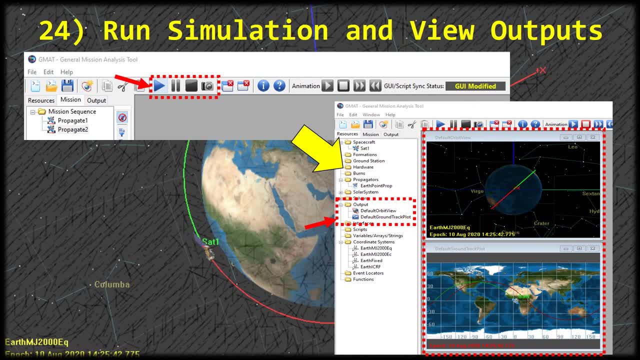 After this simulation has finished running, we're actually able to animate the results to see the satellite travel over the ground track plot or to see the satellite orbit around the Earth to visualize the mission sequence. And we'll check that on the next slide. But real quick, there's also here on the top right this GUI modified. 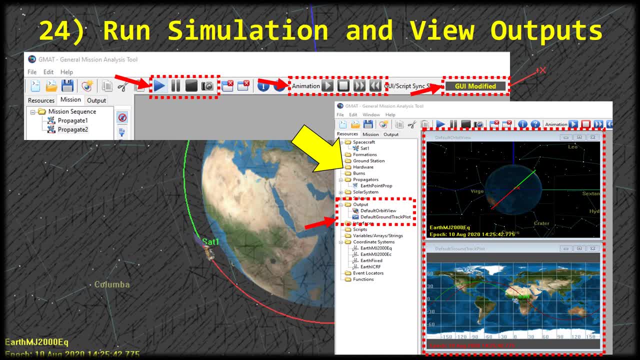 This simply means that you've made changes to the script file using this GUI, but you haven't saved it yet. So before you close out of any of this, after you're done checking out the results, make sure that you save it, if that's what you're wanting to do. 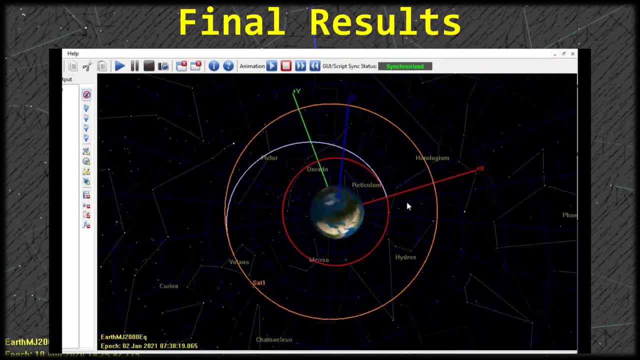 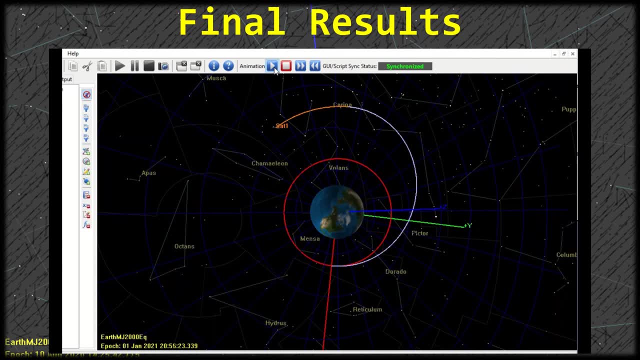 All right, let me go ahead and pan around and zoom on this 3D plot just to try and get the overhead shot make it easier to see, And then I'll hit this animation button a few times, But this is the final plot that we're going after. 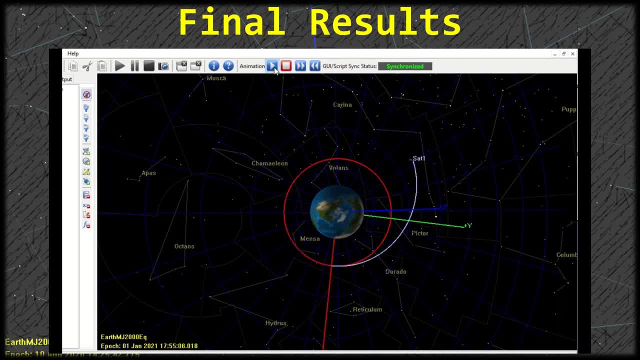 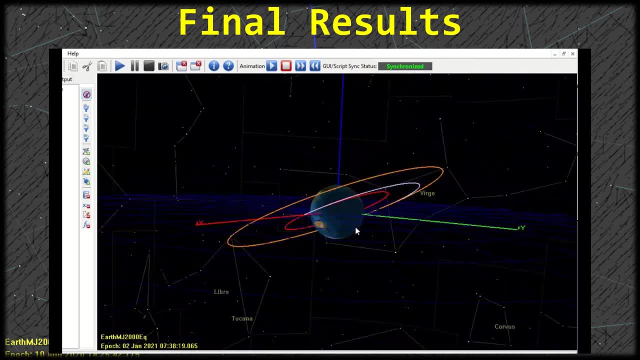 It's the same as that plot there on the left, And so it's really cool that we're able to add these burns in and be able to go from one orbit to transfer orbit To the next orbit and be able to model this Hohmann transfer. 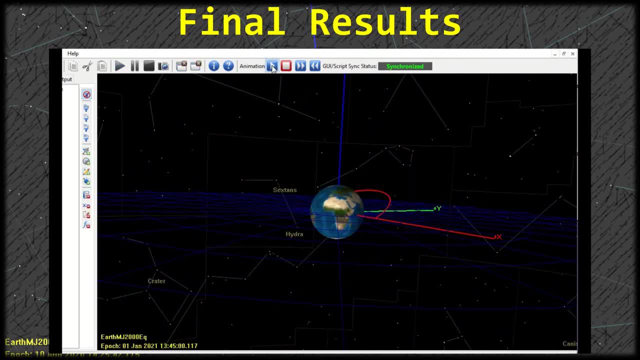 And, of course, if you like the video, thought this was a good tutorial and you want to see some more tutorials, don't forget to like the video. That's how I know that they're good and that you want to see them. All right, thanks for watching. 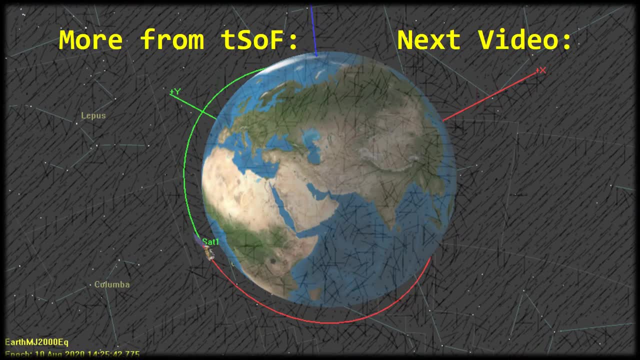 I'll catch you in the next video. Bye.